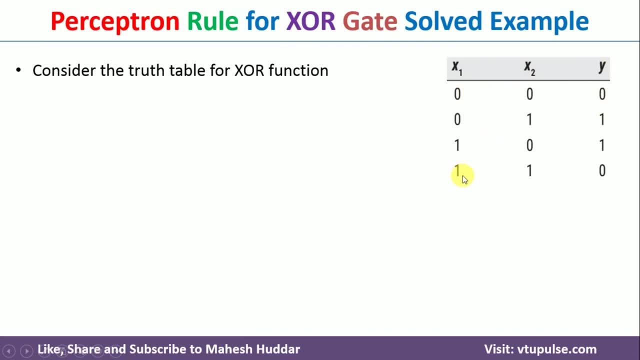 The output is low only when both the inputs are low or both of them are high. in this case, The same thing can be represented something like this: If both of them are low or high, the output is zero. If either of them is high, the output is high. in this case, If you want to classify this, 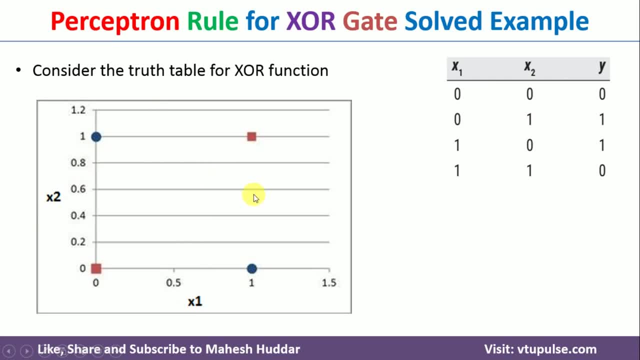 particular data with the help of a linear line, or you can say that the straight line- it is not possible. For example, if I draw a line over here, I am not able to classify this particular data properly. Similarly, if I draw a line over here, again I am not able to classify. 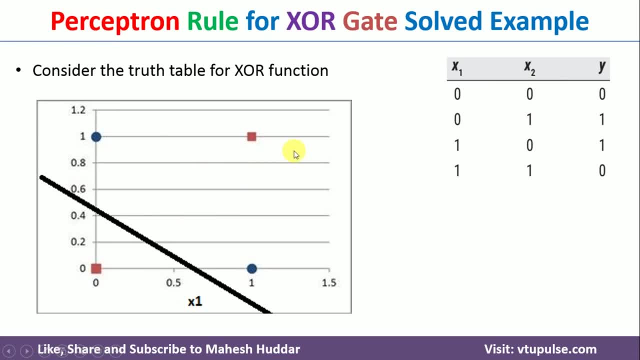 it. So this is one peculiar logical gate where the data is non-linearly separable in this case. Hence we cannot use a simple perceptron rule to find, or can say that implement, this XOR gate. Hence we will use this particular equation, that is: y is equal to x1. negation of x2. 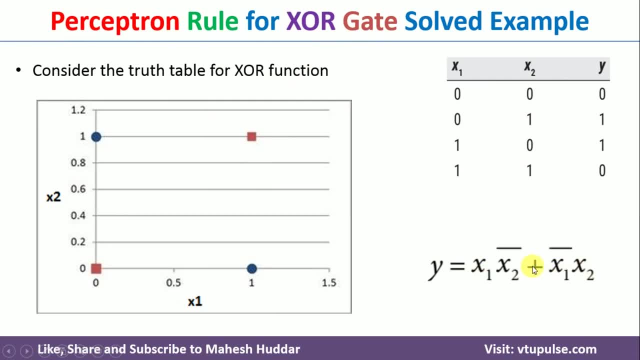 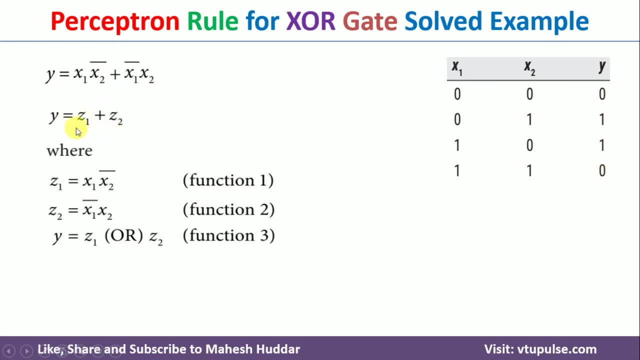 plus negation of x1, x2.. So this equation will give you this particular output over here. So what we do here is starting from this particular equation. we will rewrite it something like this: y is equal to z1 plus z2, where z1 is this particular part. That is the first part. 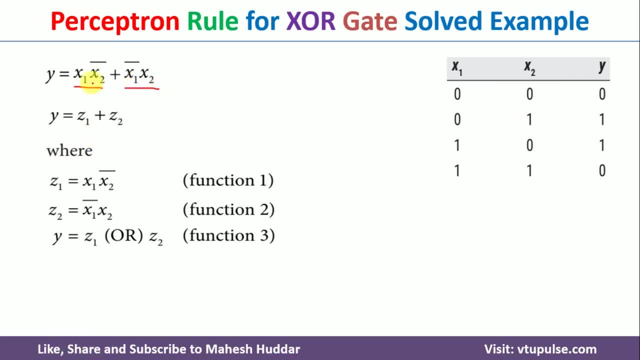 And then z2 is equal to this part. Once you get z1 and z2, we will combine them and then we will get what we can say, that the final y over here. So first we need to solve this particular z1 and then z2.. We need to combine them so that we will get this particular y over here. 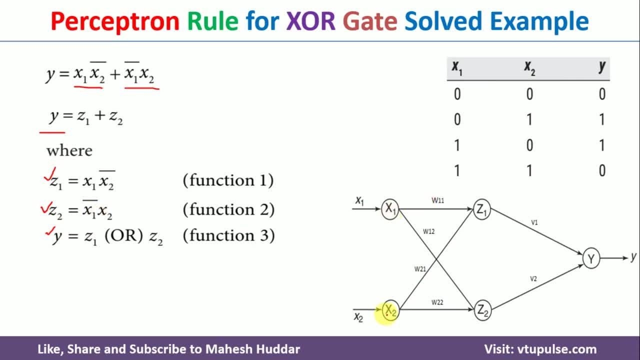 So this is how the final network will look like. x1 and x2 are the two inputs, z1 and z2 are the intermediary perceptrons, you can say, and y is the output over here And these are the weights. 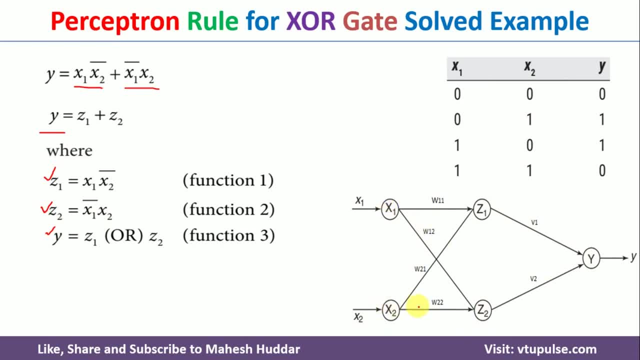 z1 and z2 are the intermediary perceptrons. you can say: and y is the output over here And these are the weights In this case. so one time we need to solve this particular side, another time we need to solve. 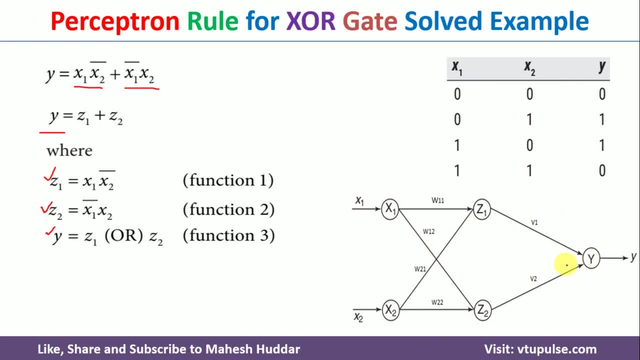 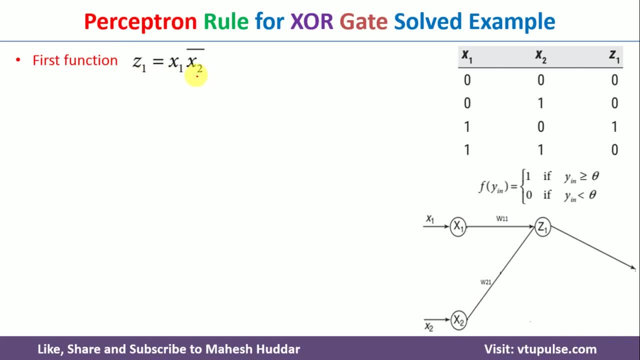 this particular side and then we need to combine it. we will get y over here, So we'll start with z1 equation. So z1 is equal to x1 negation of x2 here. So if it is equal to one and if it is, 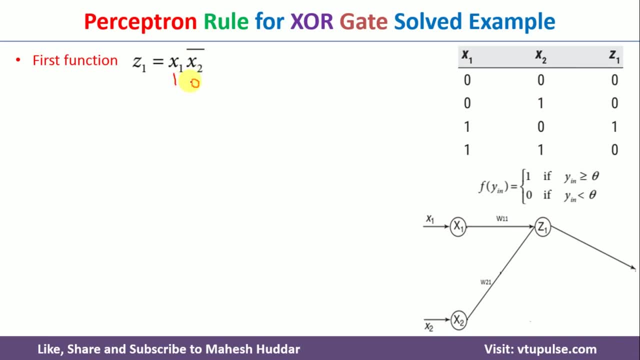 equal to zero. that is negation of zero- will become one, So one and one is equal to one over here. So only in this particular equation the output is one. in all other cases it is zero. here This is the activation function. 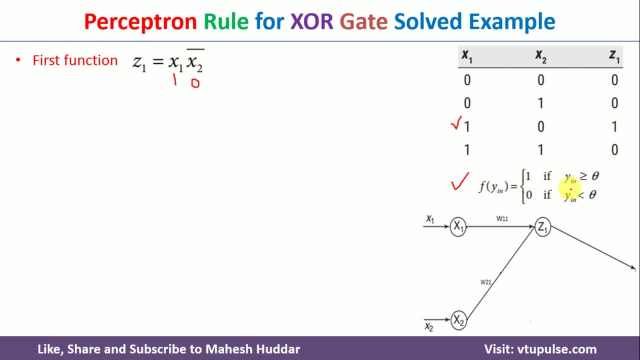 This is the activation function. If the value of, or the net input is greater than some threshold value, the output is one. otherwise it will be zero here. So we need to calculate the net input here. If it is greater than threshold it will be one, otherwise it will be zero in this case, 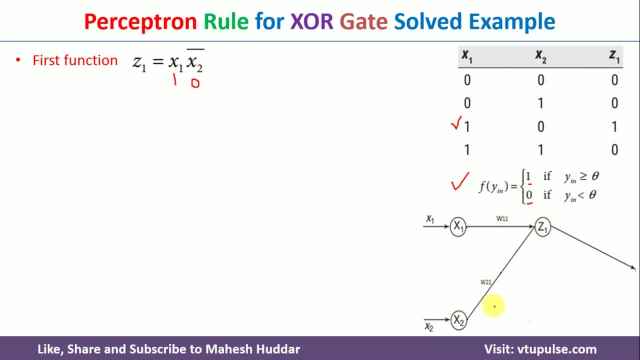 So this is for z1. And then we need to calculate it for z2 at the later stage. Now we need to initialize some of the variables, that is weights here, w11 and w21.. I have initialized it to one. you can initialize it to anything, it is not. 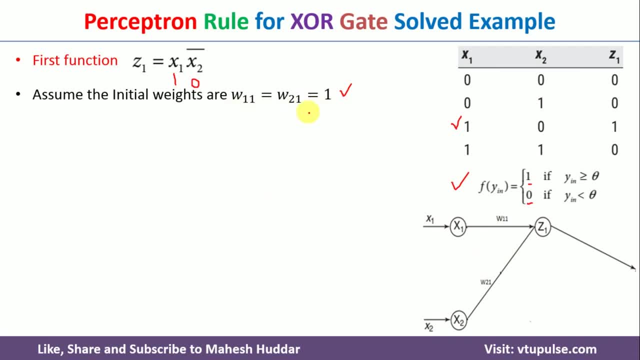 hard and fast all that. we have to start with one. we need to randomly initialize these particular weights here. Similarly, we need to initialize two more variables. The first one is threshold. you have to set some threshold value because we are going to compare this net input with the help. 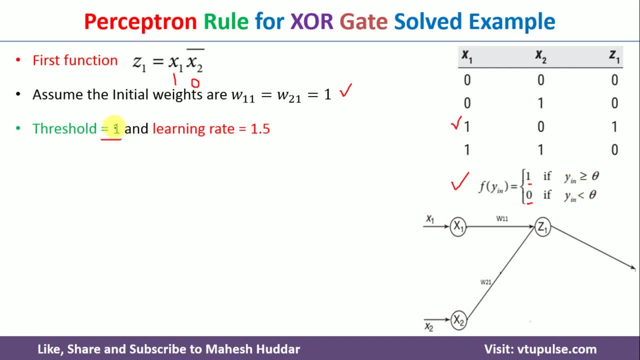 of threshold here, So we need to initialize it randomly. I have set it to one in this case. Similarly, we have to set the value of learning rate. For this particular example, I have considered 1.5,. you can consider anything again here. Now I will start with the. 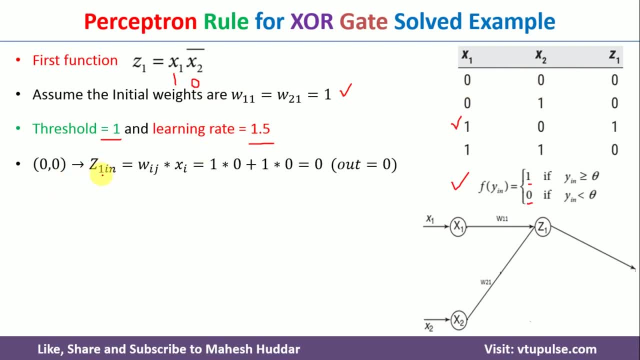 first input, that is this one, 00,. the net input, that is z1 in, is equal to wij x1. So wij is w11 in the first case. second case it will be w21,. xi is x1,. second case it will be x2.. 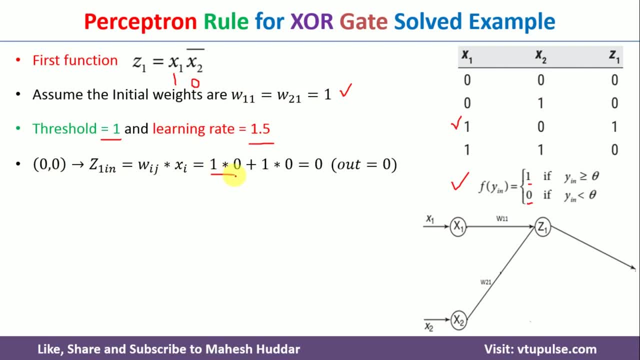 So this one is one here. So one into zero. that is the first part, And this one into zero is the second part. over here we will get zero as the net input. So this net input is the theta is one here. It is not greater than one. So because it is not greater than one, output will be zero here. And 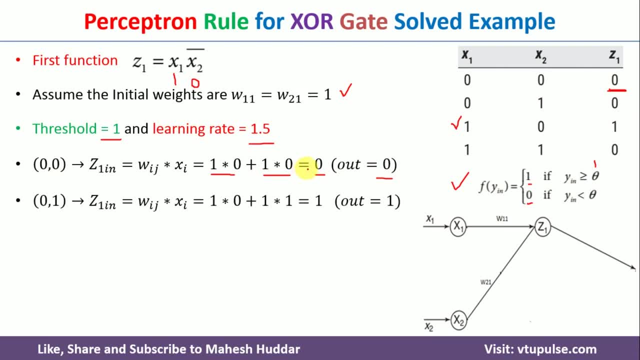 expected is also zero here. No issues in this particular case. Now I will start with the second input, that is 01.. Again, I will put in this particular equation: I got the value as one as the net input. this net input is greater than or equivalent to one in this case. So because of that, 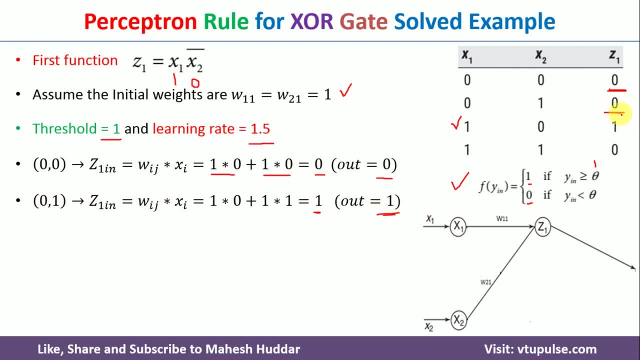 output is equivalent to one, but the expected answer or the target answer is zero here. Because they are not same, we have to update this particular weights. To update that particular weights we have to use this particular equation: wij is equal to wij. that's a old weight, plus a learning rate into t minus o, that is target minus. 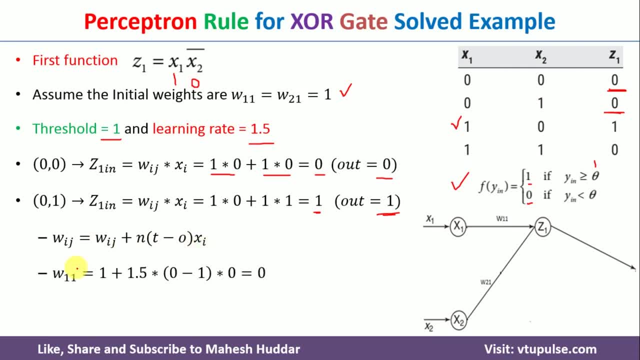 calculated output into input here. So w11 is equal to w11, that's. the previous weight was one. that is what I have written here. learning rate is 1.5, t minus o. t is what target, that is zero. calculated output is one here. So zero minus one multiplied by xi. xi is what in the 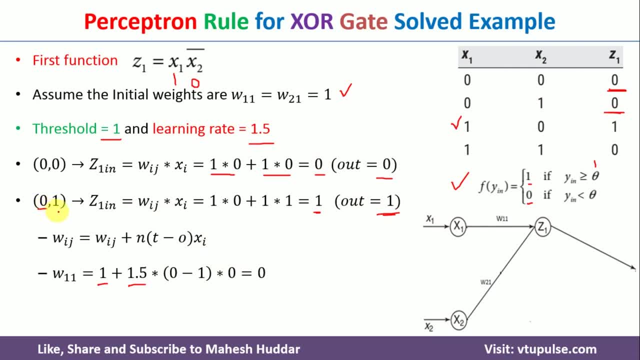 case? that's first case. x1: is this one second case? it will be one here. So if I solve this particular equation, I will get zero as the answer here. Now coming back to w21, that's a second weight. 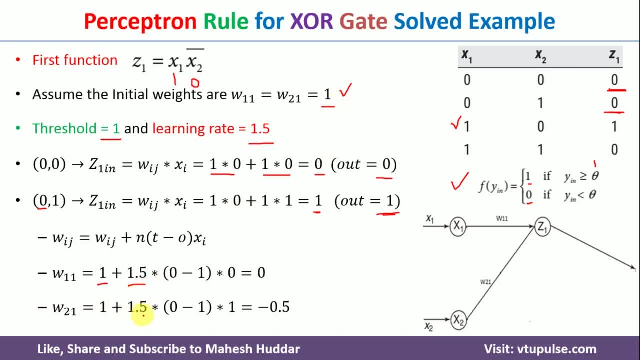 this one is one here. previously it was one, so I have written one here. 1.5 is the learning rate, zero minus one is the target, minus calculated output and input. what is the input now? this is one here. So if I solve this one one plus 1.5 into minus one, so that will become 1 minus 1.5,. 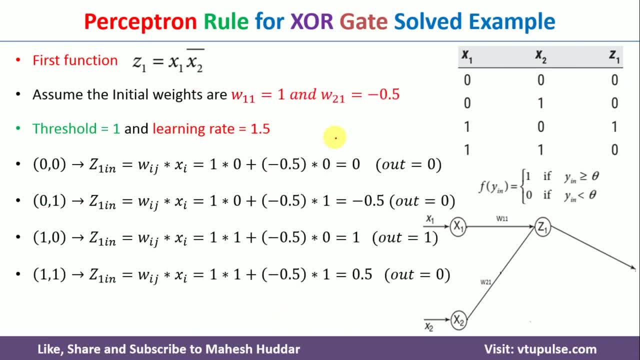 so it will become minus 0.5 over here. So w11 is one only, but w21 has been changed to minus 0.5.. Now I will start with the first input here. this is the first input, and then I will calculate the z1 in. z1 in is equal to same equation here, wij xi. 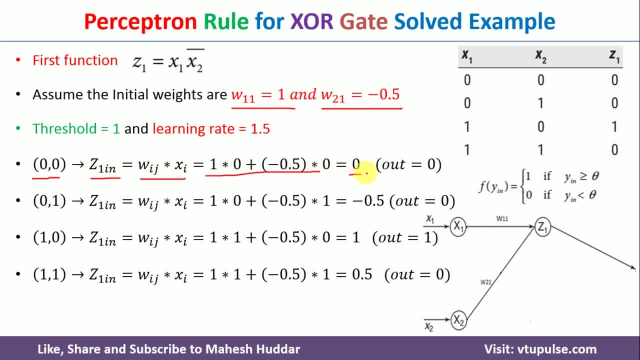 if I solve this particular thing. I got zero as the net input, because net input is not greater than the threshold, that is, it should be greater than one because it is not greater. we got the zero here and expected is zero. no issues. I will start with the second input. if I put all the 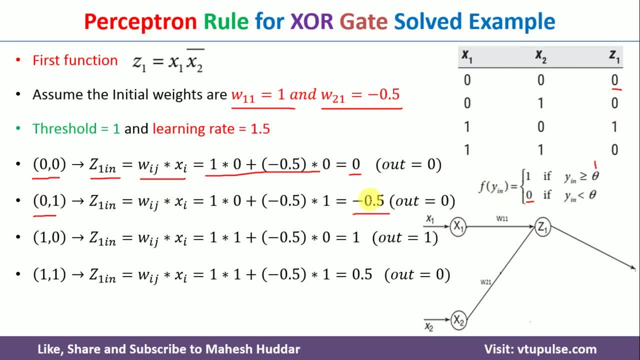 values in this particular equation. I got minus point five. this minus point five again, it is not greater than one. because of that, I got output as zero. again, it is similar to your target, so there is no need to do the weight updation. I will consider one zero. 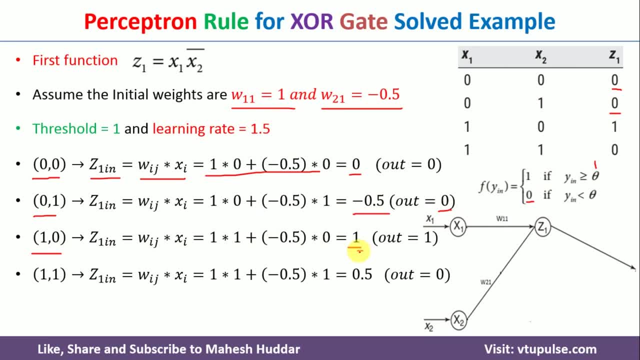 and then, if I put all those things in this equation, I got one as the z input or a z in now input is greater than or equivalent to 1, so 1 is greater than equivalent to 1, so the output in this: 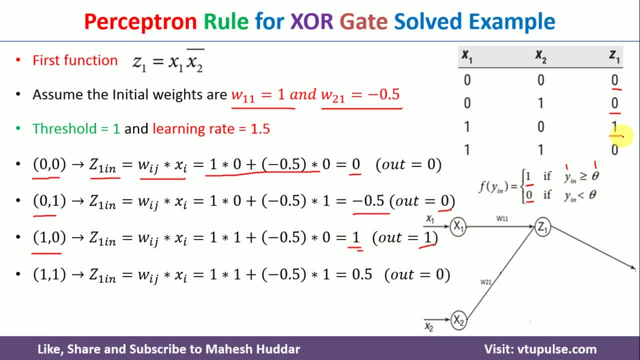 case is 1, and what is expected here? the same thing is expected. i will continue the next input, that is 1: 1. if i put everything in this equation, i will get 0.5. so 0.5 is not greater than 1 because it. 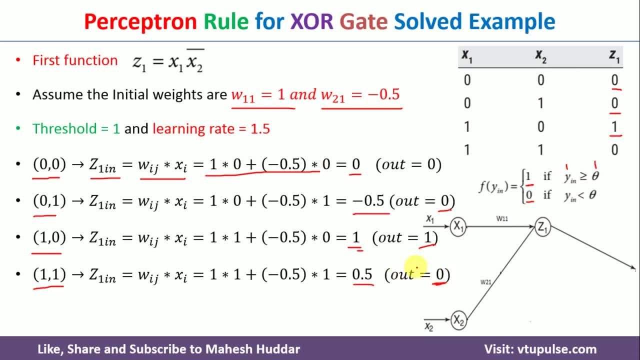 is not greater than 1. output is 0 here. so you can say that all these particular examples were correctly classified with the help of this particular weights, that is, w 1: 1 is 1. w 2: 1 is minus 0.5. threshold is 1. learning rate is equivalent to 1.5 in this case. now we will. 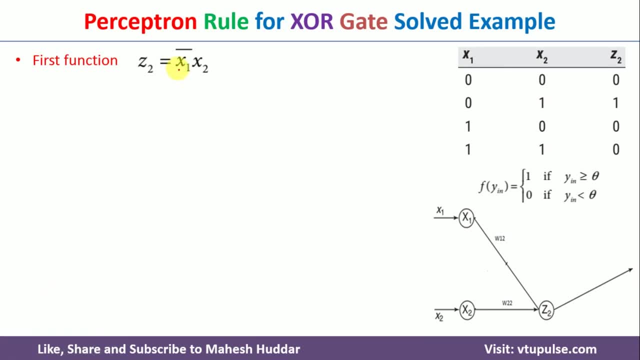 continue with the next function, that is, z 2, which is equivalent to x 1 bar x 2, or negation of x 1, x 2. in this case, the two table for this one is shown over here. if the first one, that is x 1 bar, if it. 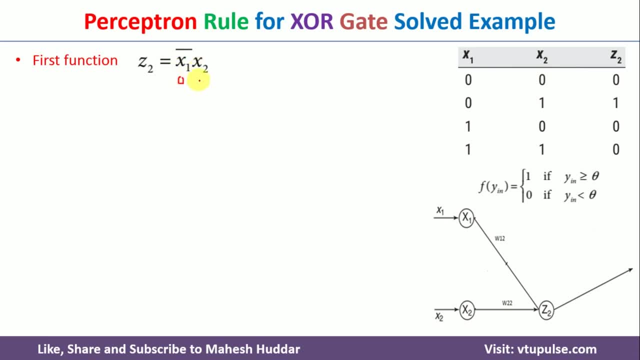 is equivalent to 0, the negation of this will become 1 and x 2 is 1. in this particular case, z 2 will become high. in all other cases it will become 0 here. so that is been shown over here. the activation function will remain same. we need to find the optimal weights for this one as well as. 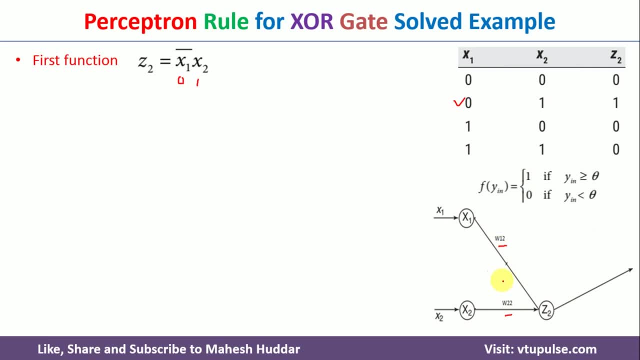 the threshold and the learning rate for this particular part of the network in this case. now i will continue with initializing the weights, that is, w 1, 2 and w 2. 2 were initialized to 1. again you can set any values randomly. we need to initialize here. threshold is set to 1 here and 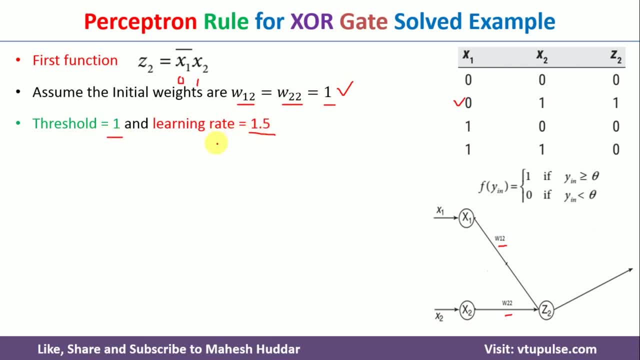 the learning rate is set to 1.5 over here. same values i have taken. i will continue with the first input, that is 0, 0. i need to calculate z 2 in. that is nothing but wij xi. if i put this particular values, that is w 1, 2 and then w 2, 2, as. 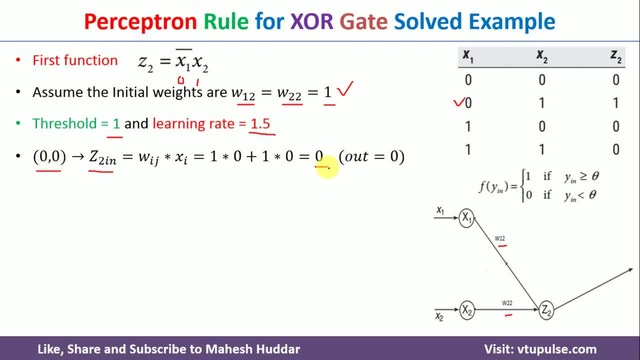 well as this input, i will get 0 as the z to in, because 0 is not greater than the threshold value, that is, 1. 0 is not greater than 1, i will get output as 0 here. the same thing is expected now. i will continue with the second input. second input is 0- 1. so if i put all those values in this, 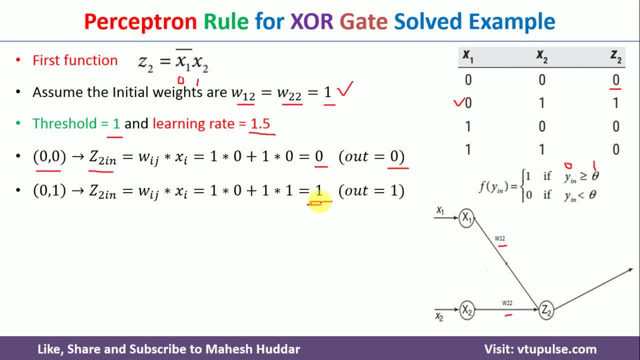 equation: i got z to in as one, i will get the z to in as 0 as the second input. and if i put z to in as 1, and because z2 in is greater than 1, here z2 in is greater than equivalent to 1- you can say: 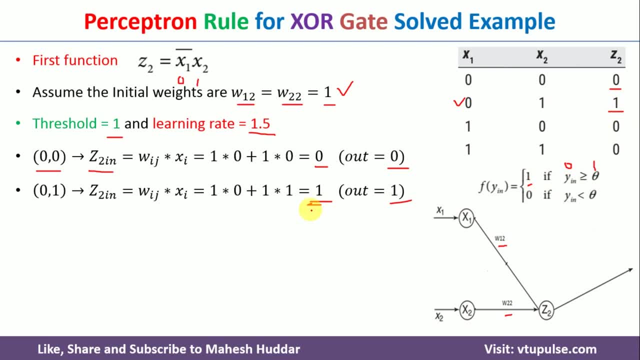 the output is 1. this output and the target is matching. again, no issues. now i will go with this particular third one, that is, 1: 0. if you look at this particular 1: 0 we got, the z2 in is 1. 1 is greater than equivalent to 1. output is 1 here. but what is expected? the expected answer is 0 here. 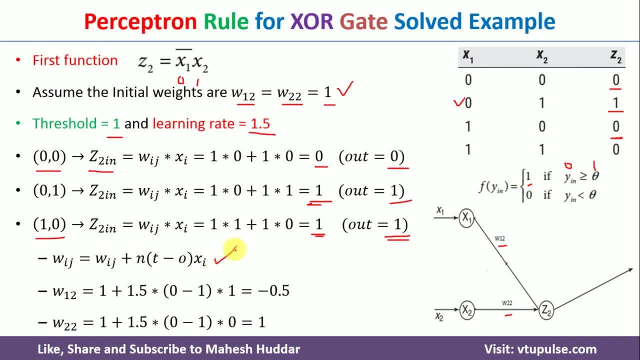 so what i need to do is i need to use this particular weight updation equation and then we need to modify these weights here. so w ij is equivalent to w ij. n into t minus o xi. w ij is known to us, that is the old weight. n is the learning rate, t is the target, o is the actual. 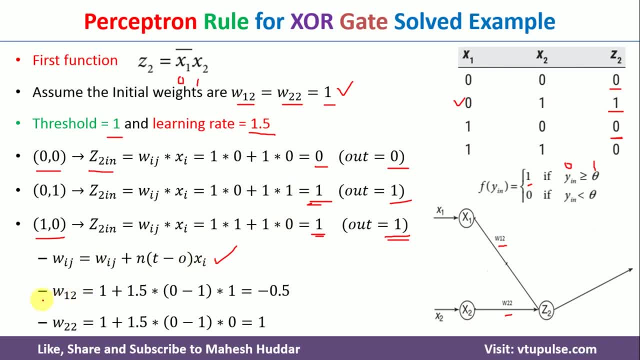 output calculated, and then xi is the input here. so put those particular things in the equations like: w 1, 2 is equivalent to 1, learning rate is 1.5, target is 0, but calculated is 1 here. so 0 minus 1 into 1 here, because this first one is 1. 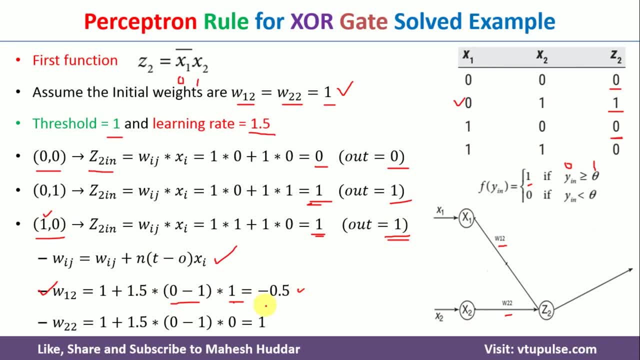 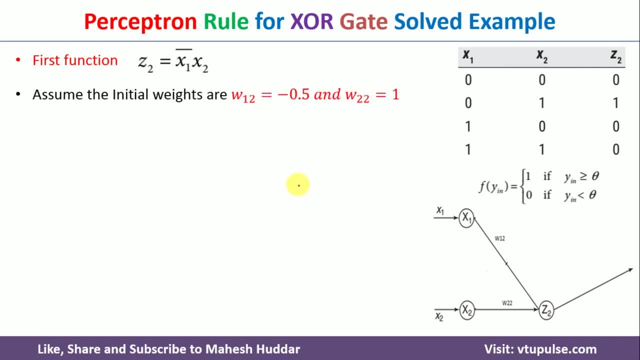 here. so we need to modify these weights here. so w ij is equivalent to w ij, n into t minus o xi. here it will become. if i solve it, it will become minus 0.5. second time this will become 0 and the answer will be 1 in this case. so we got the updated weights. that is, the first one is minus. 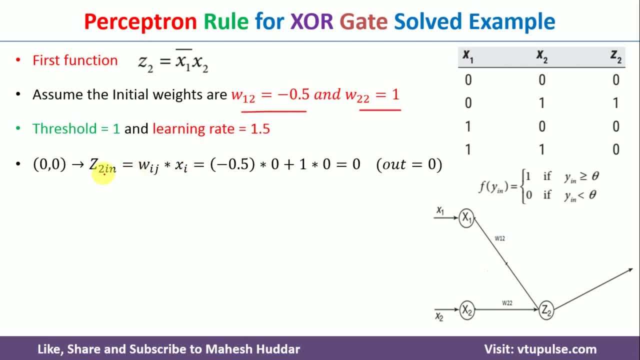 0.5 and second one is 1. here now we will put these particular inputs again. if i put this particular 0, 0- i got z2 in- is equivalent to 0, which is not greater than equivalent to 1 here. so the output is 0 here. that's perfectly fine and that is what is expected when i continue with. 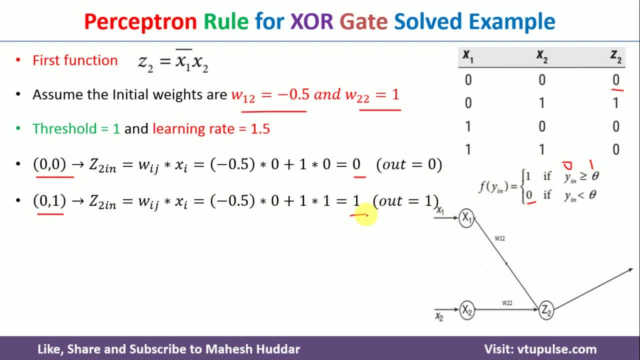 0, 1, uh 0, 1. if i solve it, i got z2 in as 1. 1 is greater than equivalent to 1. because of that, i got 1 here. 1 is the output and the target is also 1 here. similarly, next time i got the minus 0.5. 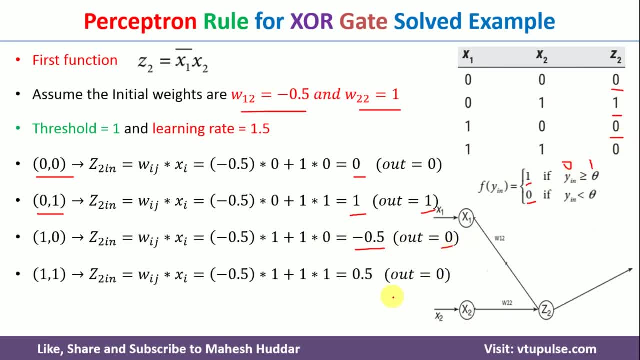 output is 0, expected is 0 here. last one is 0.5. again, 0.5 is not greater than 1 here, so output is 0 and expected is also 0 here. so with respect to these weights, i am able to classify that. 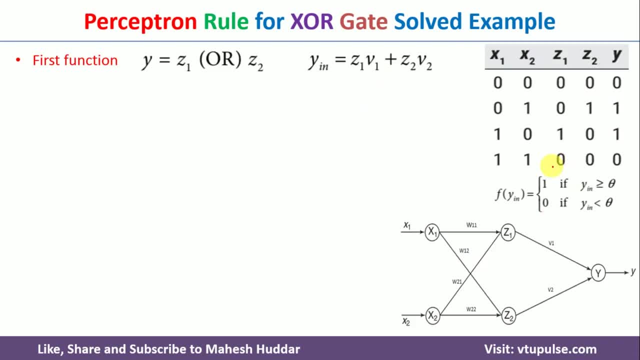 data correctly in the future. so this is the output, and this is the output, and this is the output and in this case also. now i will continue with the next one, that is, y is equal to z1 or z2. z1 is known to us, z2 is known to us. if you go back and see this particular thing, z2 is equal to 0 1 0, 0. 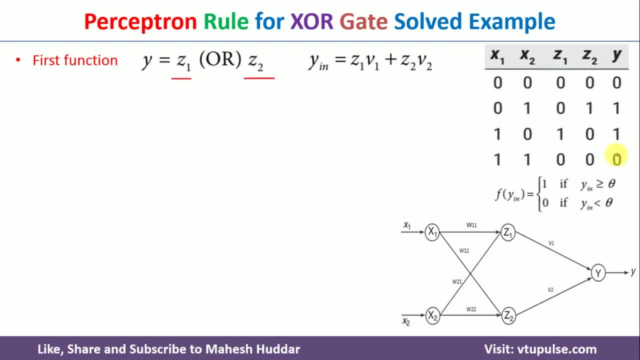 z1 is 0, 0, 1, 0, that is what we have already calculated. so z1, i have written here, and then z2, i have written here- y is what y is, or between z1 and z2. that is, this one is 0, this one is 1. 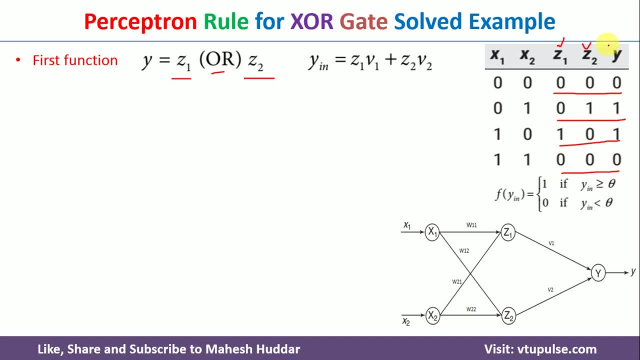 this one is 1 and this one is 0 here because or will be high one. you can say that if any one of those particular input is high, in this case both are low. in this case also, both are low. so we have to consider this particular input and then we need to find out the value of v1 and v2 here. 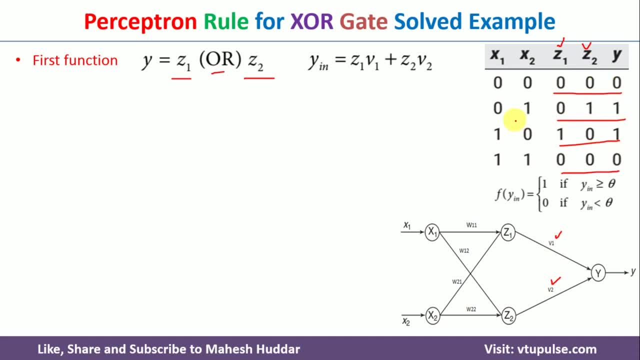 these are the inputs and these are the and this is the output. and if you look at this one with respect to x1 and x2, we are expecting the same thing here. if these two things are there, we are expecting one over here. Now again. 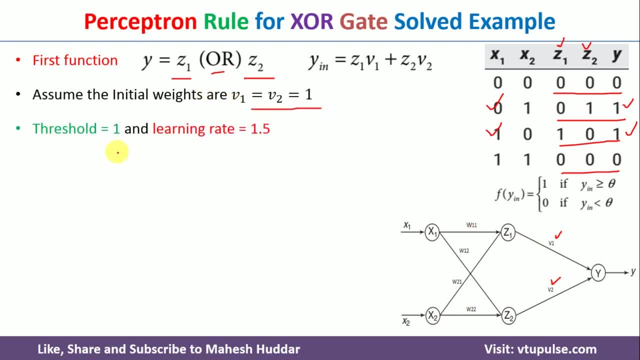 we will initialize these two weights, that is, v1 and v2 to 1. here threshold is one, learning rate is equal to 1.5. i will start with the first input. i got v1 in as, or you can say y in, actually, y in. 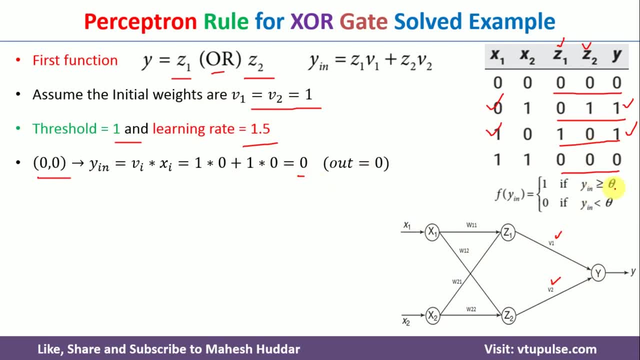 is equal to 0. 0 is not greater than threshold, that is 1, so the output is 0. expected is also 0. here continue with the second one. i got y in as 1. 1 is greater than equal to 1, so the output is 1. 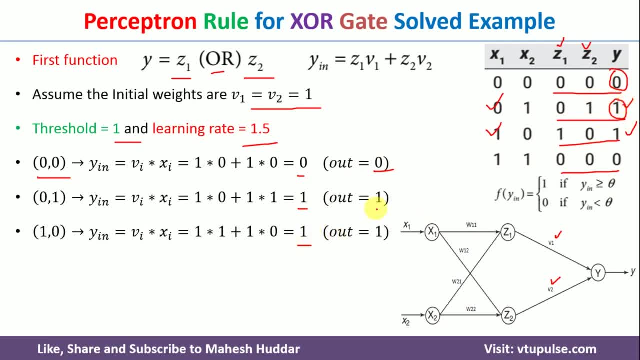 target is also 1 here. coming back to the next one, the next one, that is 1: 0. you can see here, this is 1: 0. i got the wine as one because it is greater than equal to 1. output is 1. the expected is also 1 here. now again, one more input is there, that is 0: 0. 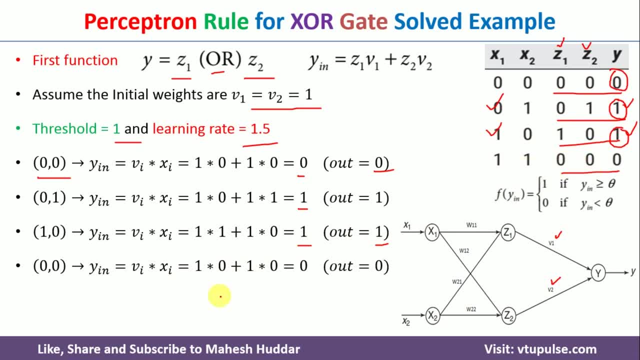 don't consider this one, because we are talking about z 1 and z 2 here. this 0, 0, 0, 0- because we have 0, 0 wine, is 0, 0 is not greater than equal to 0, so the output is 0 here, which is as expected. now, 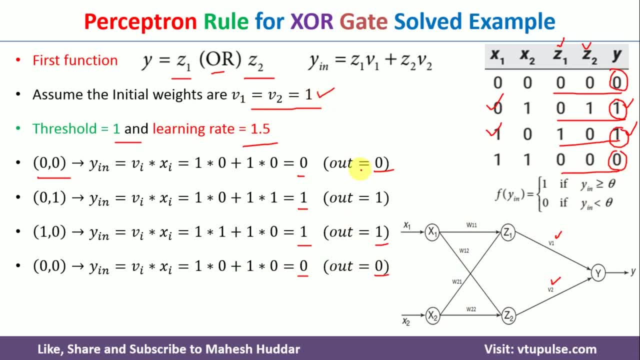 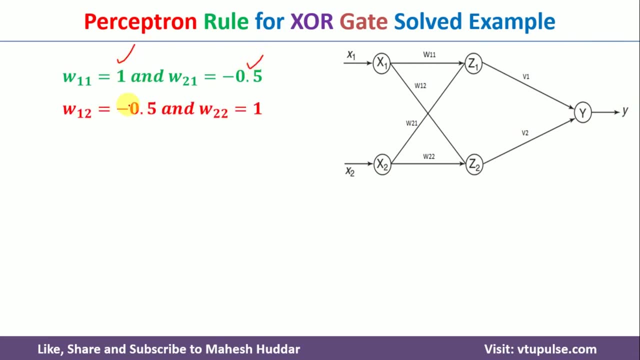 with respect to 2, v1. and v2, that is, if both the values are 1, we were able to classify this particular data successfully. so that is the final weights for v1 and v2 for this particular threshold and learning rate. so finally, we got w11 as 1, w21 as minus 0.5, w12 as minus 0.5, w22 as 1, v1 and v2 as 1 in this case.